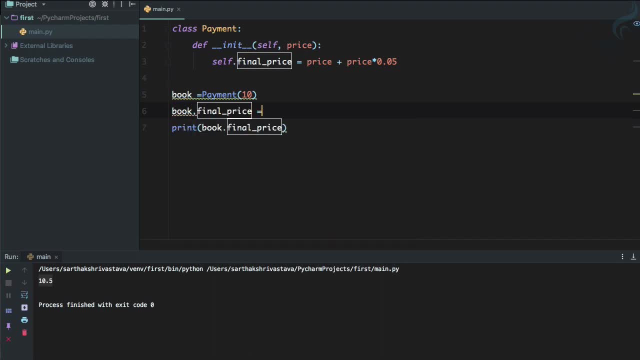 If someone do this book dot, final price is equal to zero. Run it And what is this? Our final price is just becoming zero. We don't want ever to do this kind of things in a big project. We don't want to do this. So how we can restrict the user to do these kind of things? So the problem here is: 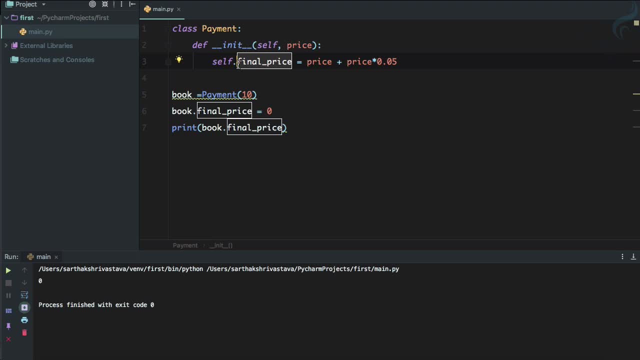 this final price variable, or the final price attribute, is actually public. Anyone can see it, Anyone can change it, no matter. whatever you want to do, Just do it because it's a public one. We need to make this as a private variable. So how we can create a private variable? 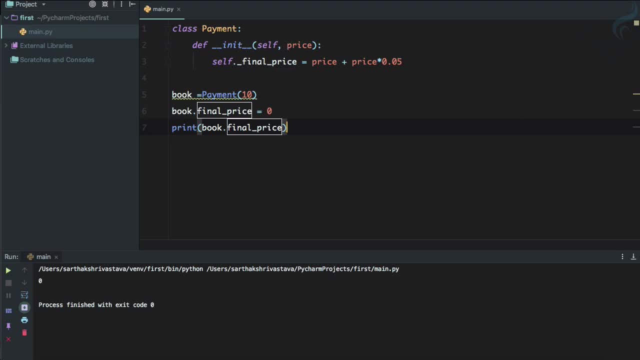 You just need to say a single underscore, But the single underscore just giving you the definition that, hey, this is a private method, You should not change it. But what if I can change it? So I say underscore and underscore, final price And yeah again. 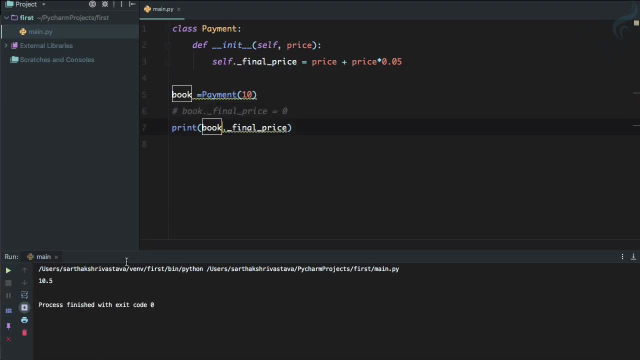 it's zero And if I'm not going to change it, yes, it is ten point five. So what's the benefit of using underscore here and making it a private? It's not looking like private. Yes, One single underscore makes a variable private, but it just it just like a warning that this is. 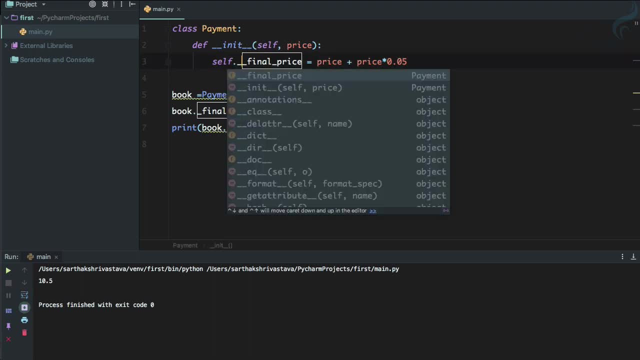 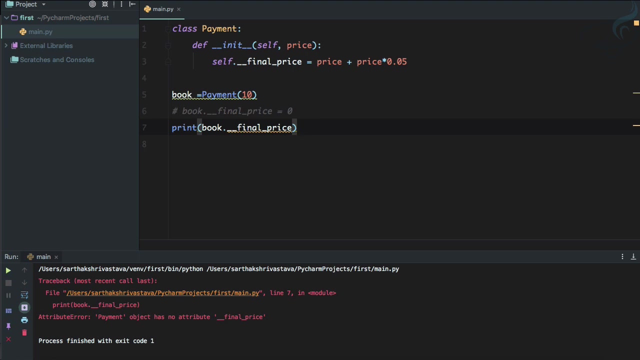 a private. But if you want to hardly say that this is a private, no one going to change it, You need to use double underscore. And now with the double underscore let's try to check this. So with the double underscore, if I try to get, you can see no one can access it. So it says actually: 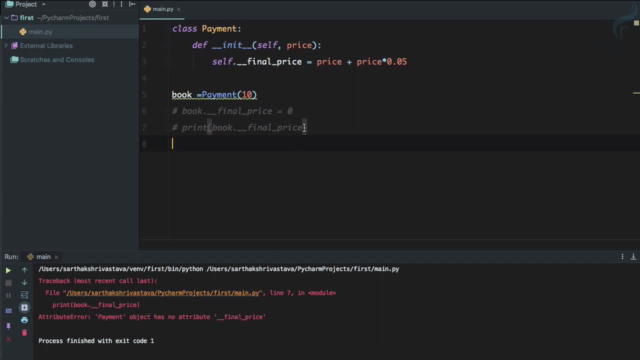 payment object: no, has no attribute called final price, because this final price is a whole private method To just this class, not for the object. But we want the price, We want to know what is the price, how we can get that if we can't access the final price. Okay, So for that you need to define a. 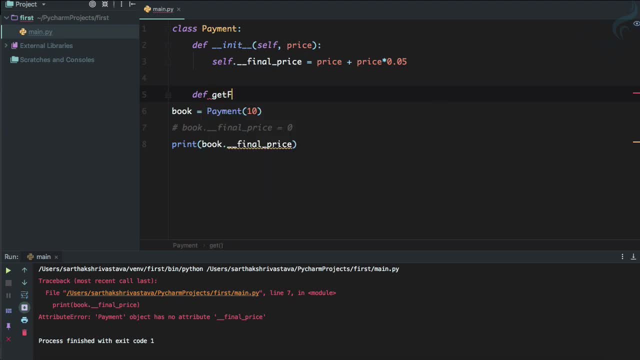 getter, Getter is just going to get final price. So I will say: get final price, And this is a function I have defined, or you can call it method, And it just going to return self dot final price. And now you can see, because we are still on the 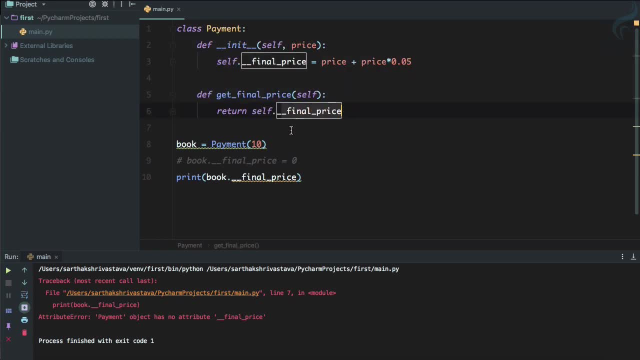 class we can access this final price variable And with this method we have returned that. So now I can say: get final price and run it. And yes, you can see, ten point five is there And even no one can change it, because if we try to change it, 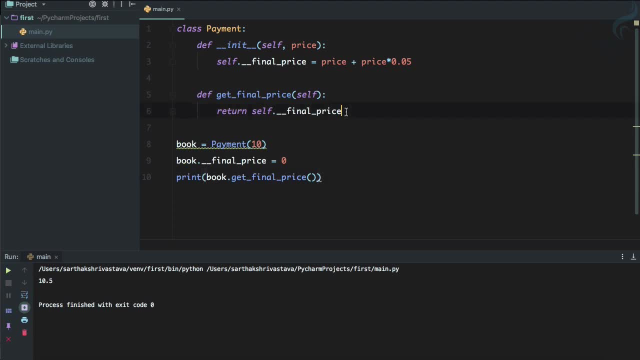 it doesn't effect because this is a private method. we have just created a wrapper to get the final price, so this is the way we can ensure that no one can change the value of this final price variable. this is good that no one can change it. but suppose you have given a coupon, so on the final price you 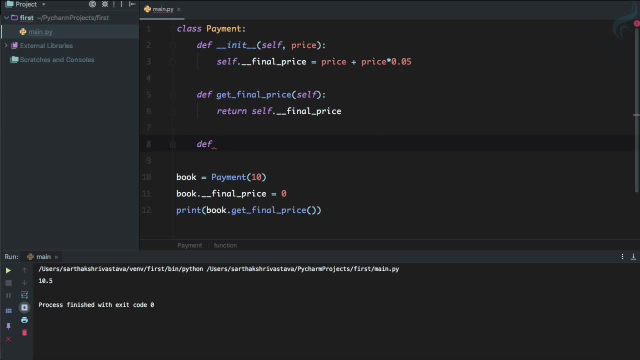 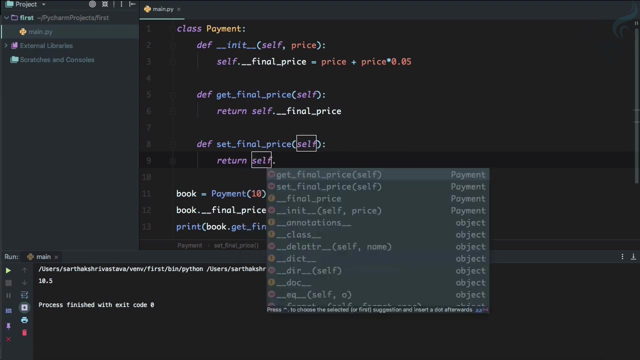 need to change something, and if we have a coupon then we need to change. so now we need to give a new method. we call it setter or set final price. so again, this is going to get return of self dot final price, and now it's going to multiply with the coupon. so let's say, or we can simply say, 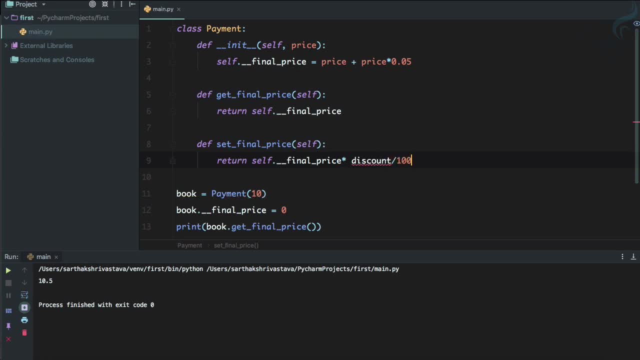 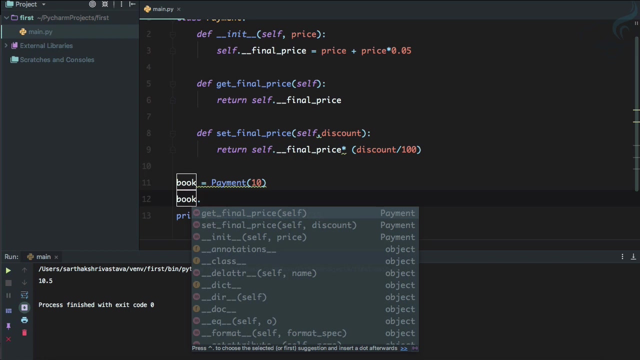 discount and divided by 100. so discount divided by 100, just making the percentage into a real value. so this is going to give us a return of self dot final price. and now it's going to multiply the value. so let's grab the discount from here and now if we want to give any discount. so book dot. 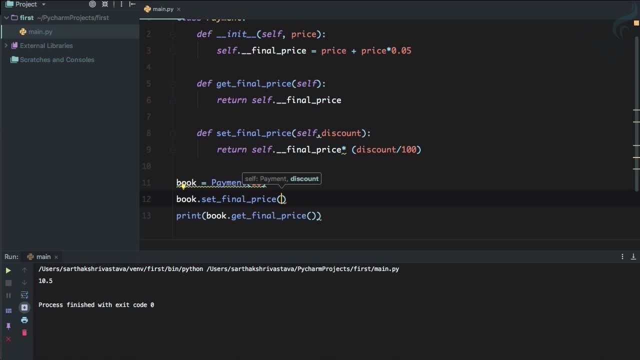 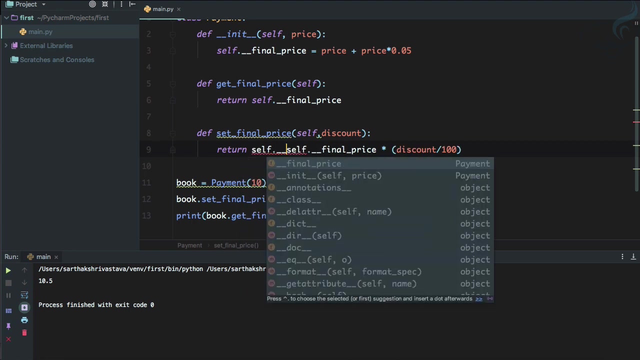 uh, we can say: set final price and giving the discount of 10. so let's see, the final price is going to be 10.5. still, okay, we are not getting that. you know why? because I need to say here: self dot underscore: final price is equal to this and I'm 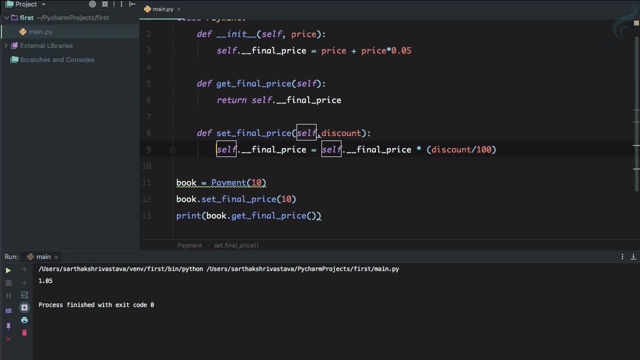 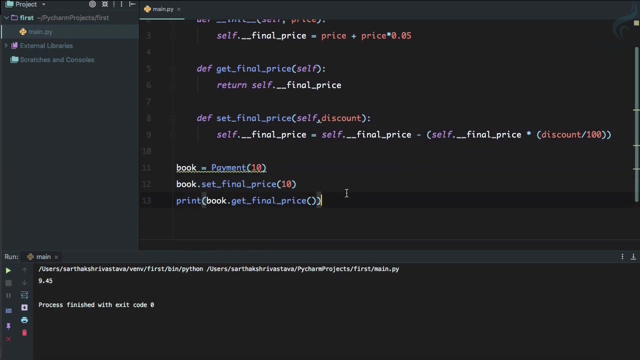 not going to return anything. so now, if I try to run, yes, you can see 1.05. we have given this much of discount which is not good. we need to say here self dot final price minus all these things. so now, if we say 10 discount, after the 10 discount, 9.45 is there. so in that way you can change. 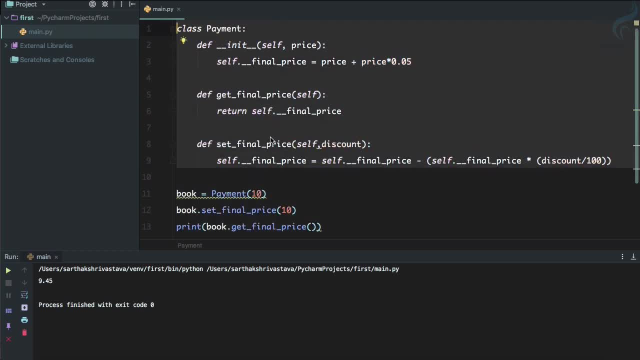 the variable inside the class, but you cannot directly change, use the variable. so this is the way python gives you private variable. in some other languages there are protected, but python doesn't have. python is very cool. it says yeah, either it has to be global or public or it's a private, nothing else. now comes the private methods. so these methods set final. 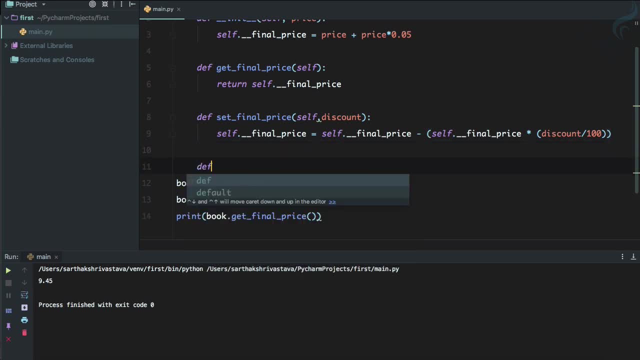 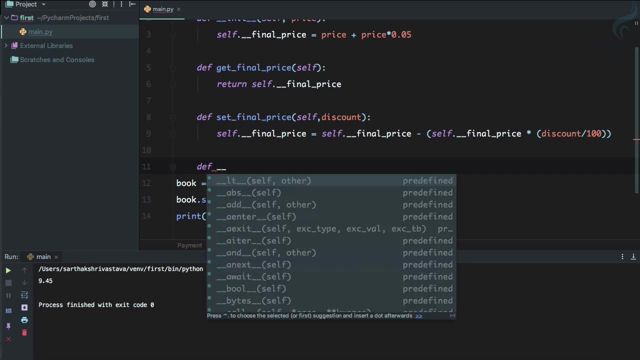 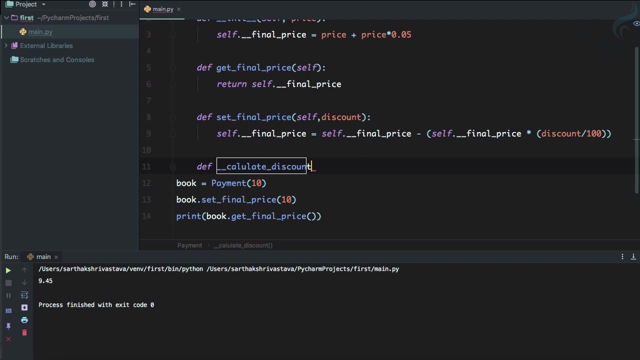 price, get final price, are public, everyone can use it. but now we can Define a private function or private method which is again using the double underscore, and I will say: calculate discount and we are going to get discount here and actually that has to be calculate, and now it's going to. 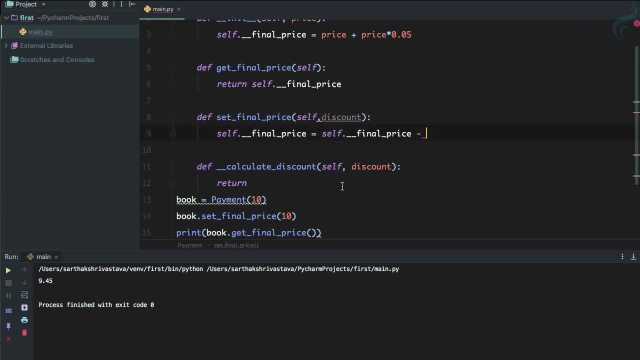 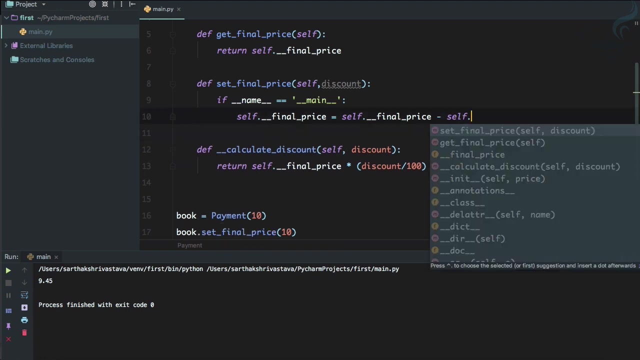 return all these things. so let's grab from here, paste it here, and we don't want this parenthesis. so self dot, price and discount, and here I will say self dot and self dot underscore, calculate discount and just pass the discount. okay, so again, if I run it, it is still going to work and no one can use this. 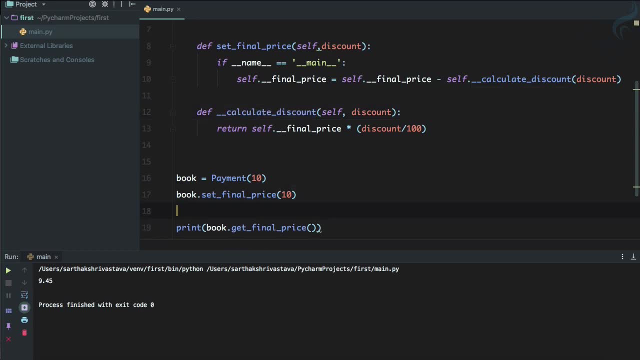 function. so if I try to use this function just after or just before set, set final price, so book, dot, underscore and so Calculate, and I am giving discount of 50 percent, let's see the result. it's going to crash because it says payment object has no attribute called underscore, underscore. 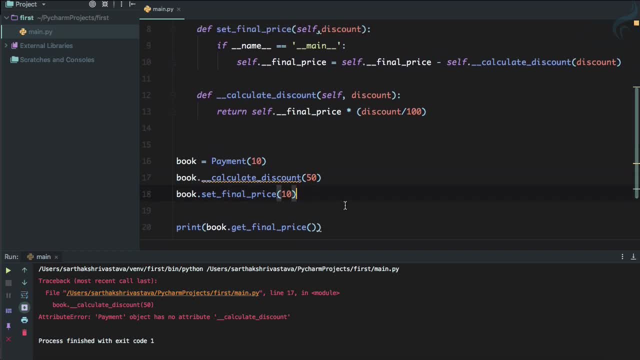 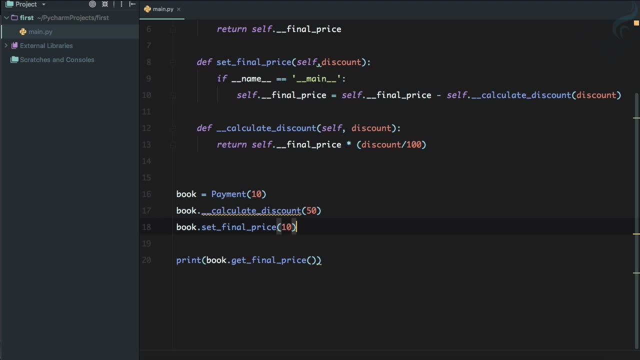 calculate discount. so this is the way you can have the encapsulation. that means encapsulating, making things private or public on the encapsulation. this is very nice and if you like this episode, please share these videos with your friends and family and I will see you in the next video. bye, bye.